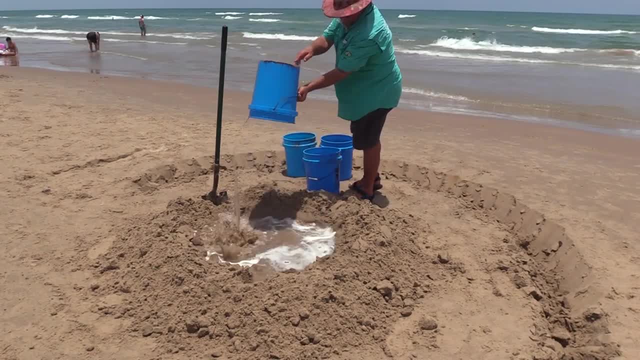 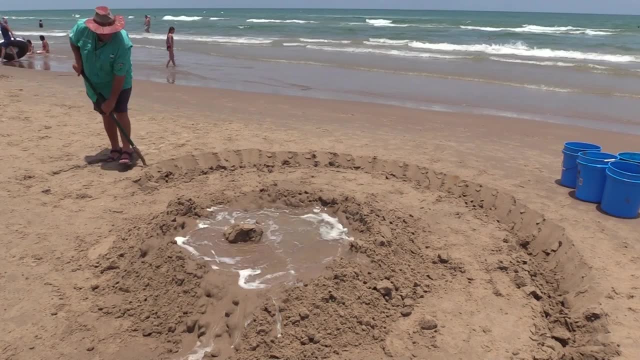 wide, so you've got enough room to stand up. but also it's very important the volcano is constructed properly. we use quite high-sided ones, from a foot all the way through to 18 inches high, and there's a lot of sand in them and a lot of water. 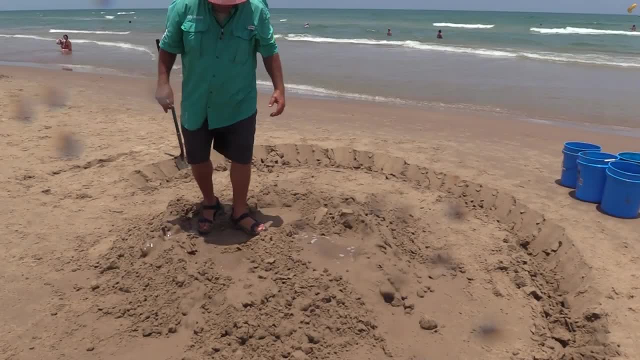 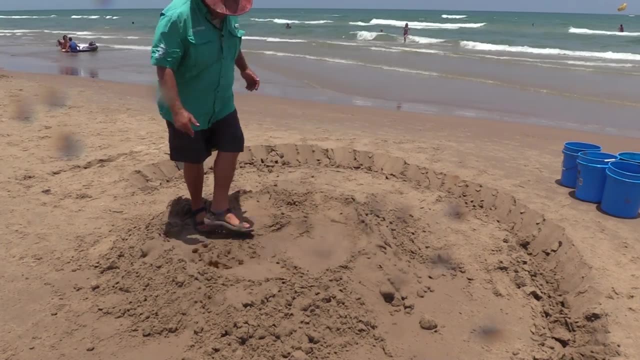 you have to stabilize it, um, with plenty of water, and then after that you can just spread it out of your feet. you know, when it's roughly level, gravity is going to level this for you. I mean, this stuff isn't a rocket science, this is just science. you know, gravity is going to do the work for you as. 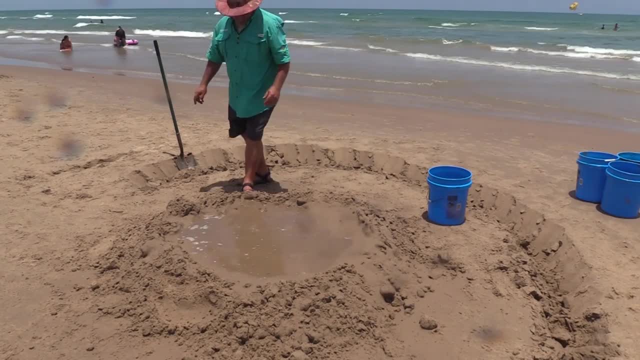 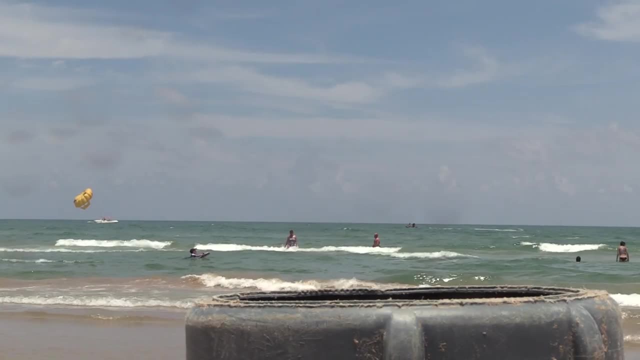 long as it's a molten pool, as you can see, then what we do is we can pack the side of our volcano, and this is important because it allows the vibration, allows the water to spread right through to the side of the volcano. that's very important, then, when we put our trash can on, when we're 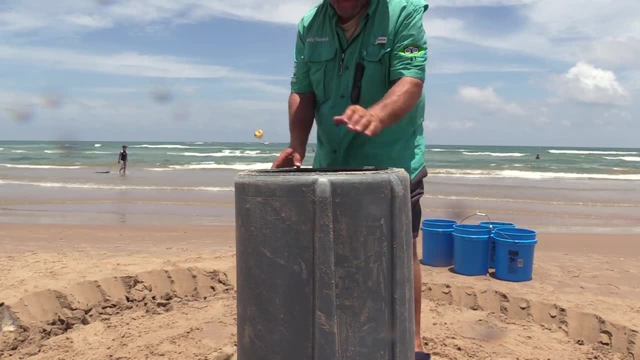 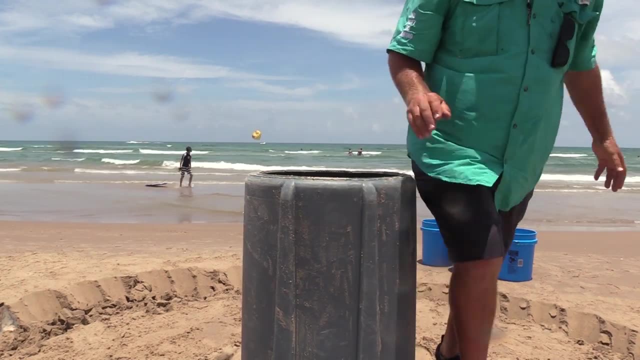 setting the base. you can see clearly from the horizon that that thing isn't straight. so we just give it a squid around. that's a good word, squidge and uh. squidge around and make it level. you can see now that it's parallel with the horizon and it's just nice and easy. the other side, we just eyeball it, you just. 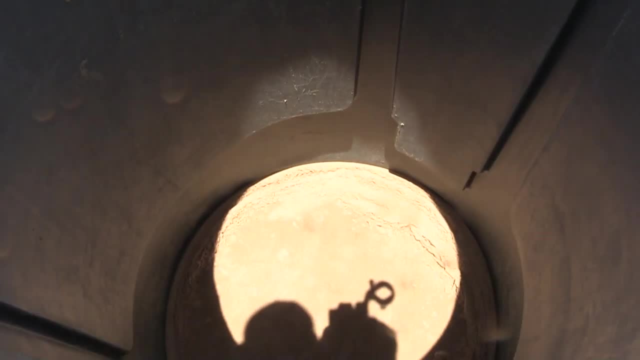 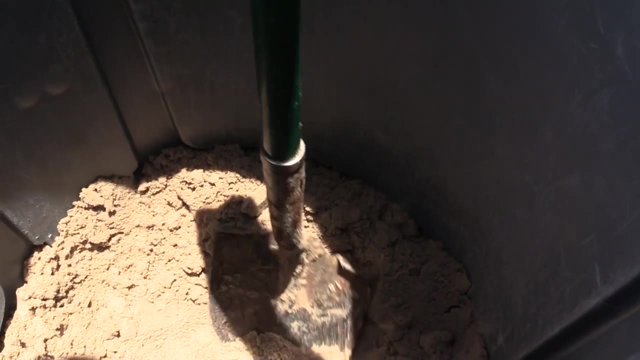 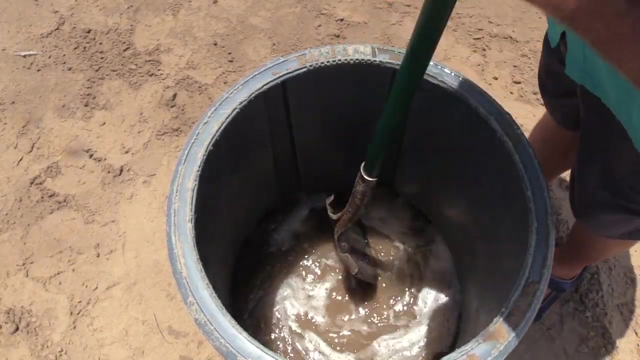 have to take your chances, really. then we- oh there we are, hello and uh, make a dish shape, put some sand in the bottom of this and make a dish with the shovel like that very simple, and then pour it in the middle so it doesn't blow the bucket out, and then chop the, chop all the sand up, and so 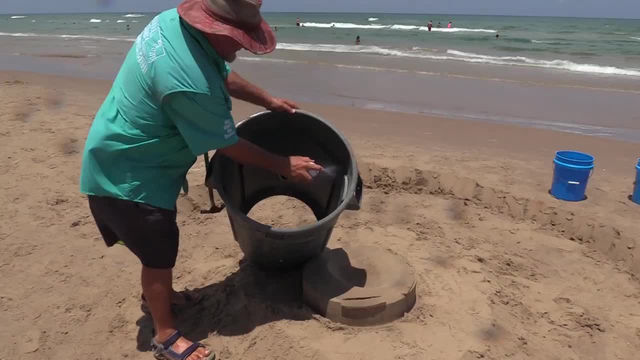 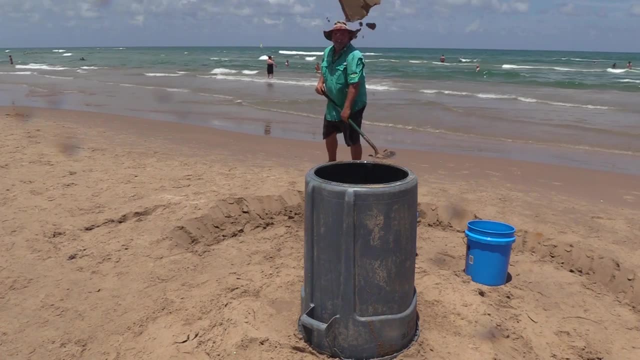 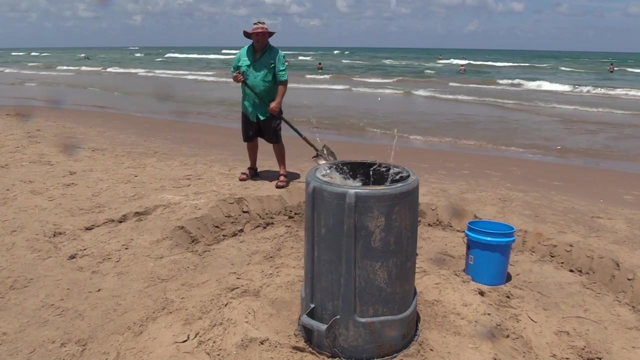 until you feel it go hard under the blade of the shovel. it's very easy. oh, and uncle Andy ding made a big mistake here. um, he didn't spray the bucket, what a Wally. so, uh, good job. I spotted it with only six inches of sand in the bottom, so I had to redo the first procedure after spraying the bucket and 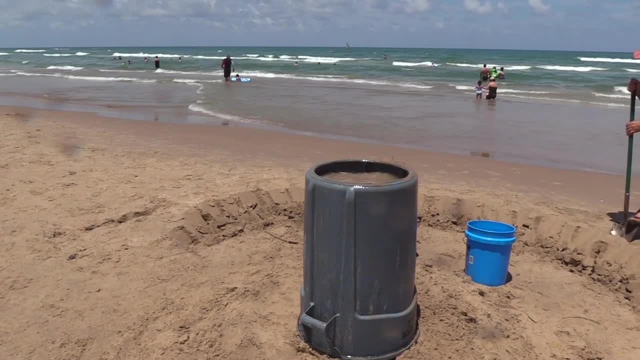 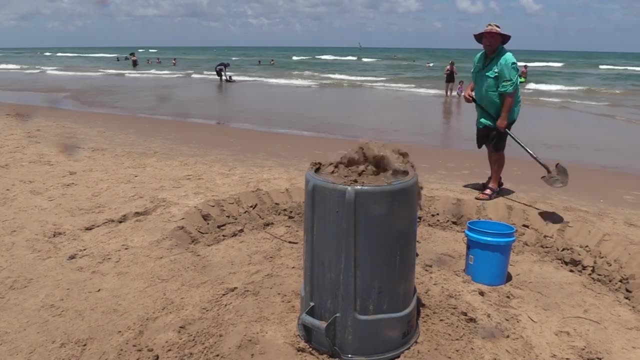 then I hurled all this sand in um, and we've speeded it up because it's very dull watching me throw sand, even though I've been told that each of the pieces turns over in the air, I didn't even notice myself. but anyway, we fill it up like this, very simple, and then spread it out with your hand. it's nice. 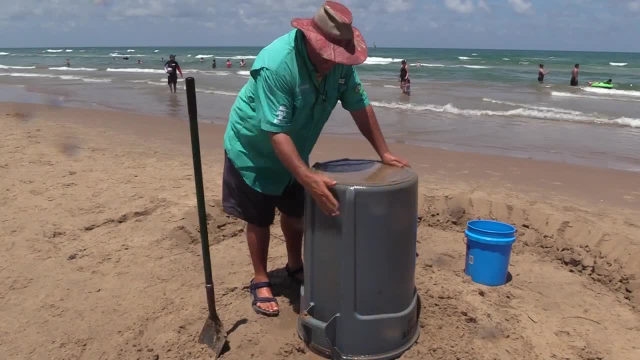 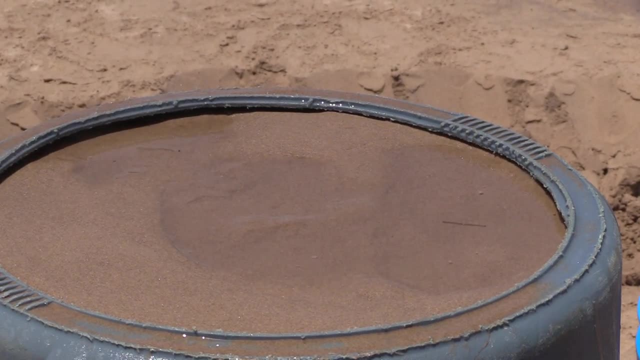 and wet, fantastic. put the shovel in the ground right and then watch the water. if the water is touching the bucket in the same spot all the way around, the water is held down by gravity. gravity makes it level. if the if it's touching the bucket in the same place, it must be level. and, as you can, 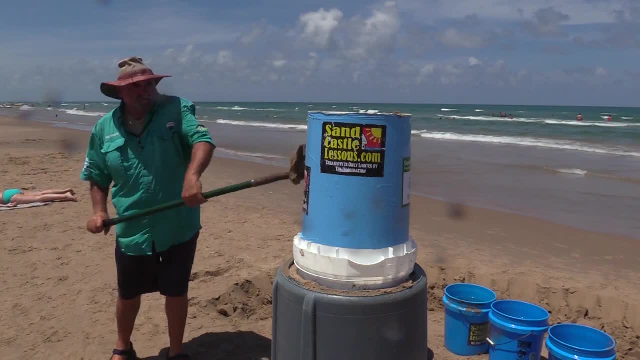 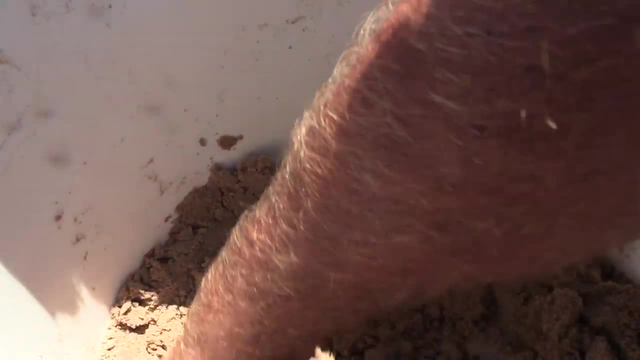 see even our Mantra: creativity is only limited by the imagination. and at sandcastlessonscom we've got a big imagination. so same procedure again: you put your bucket on, put some shovel, shovel about a third of the the size of it with sand, make a dish with your hand and then pour the water in. really, 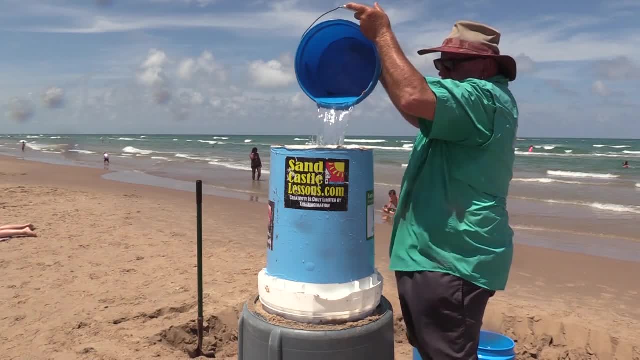 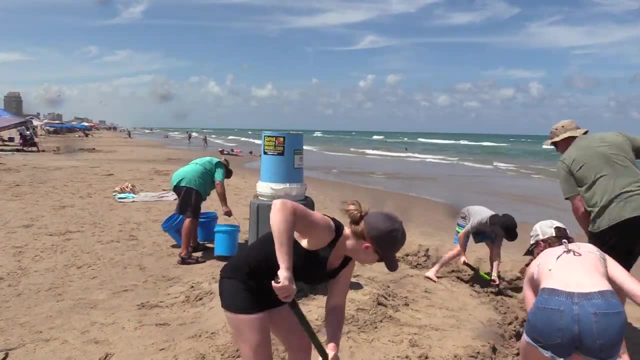 really simple. it's. this isn't, like I said, it's not rocket science. then you vibrate the bucket. you tap the bucket all the way down, the same as you would have done with the shovel, and tap, tap, tap, tap, tap. you introduce that vibration when you put the. 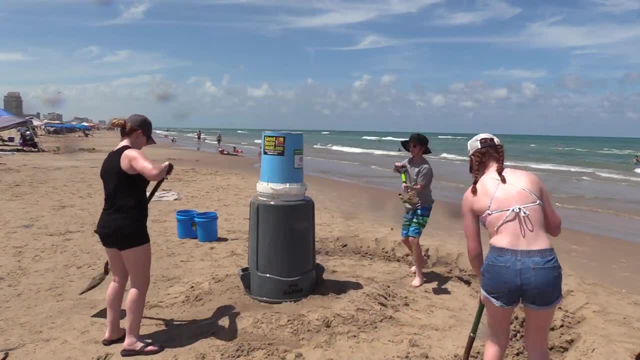 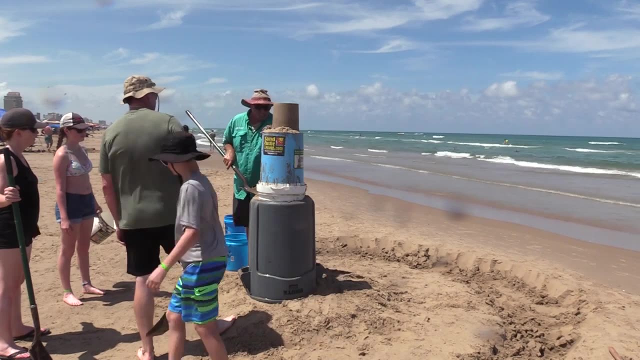 bucket on. see everybody's shoveling it sand to water. that's another important point as well. you always put sand to water for two reasons. number one: it takes all the air out of the sand, which makes it a lot stronger and introduces compaction and granulation, and then also it lifts all the 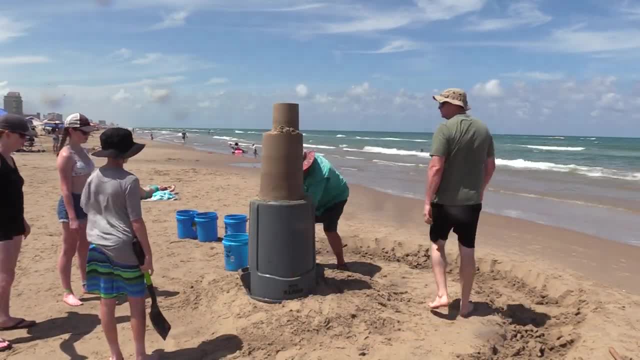 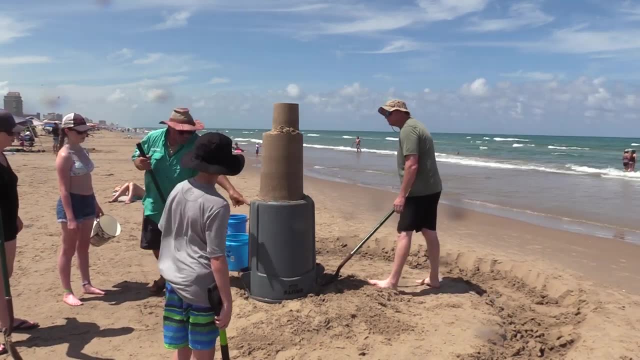 trash to the top of the bucket, which means you don't. it's like self-cleaning sand, so if you've got a beach that's a bit dirty with seaweed or trash or whatever, all the lightweight stuff will float on the water. so it means you can get it out of the way. uh, and then when you take in the big 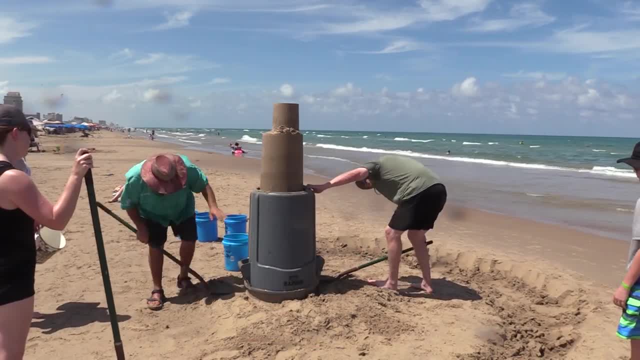 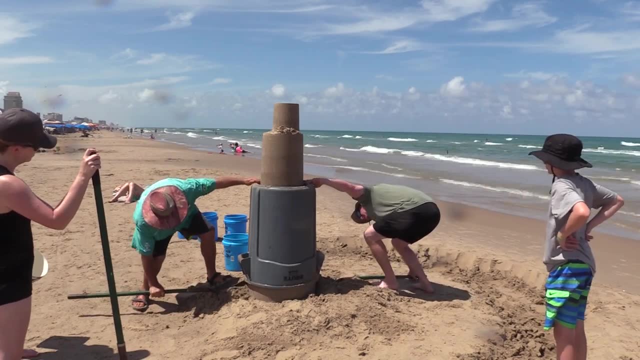 bucket off. you have, there's two of you. this needs two of you. you can't do it? well, you can do it by yourself, but it's very tough, um, and basically you have to use that shovels as levers and then gently bounce the shovel. you can see, we've speeded it up for this. 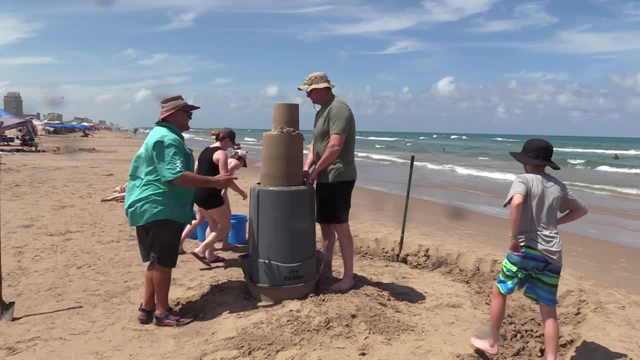 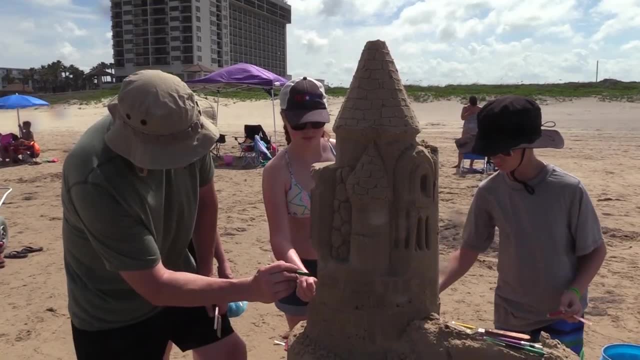 but you're actually bouncing the shovel, um, and this family can stand around all they want, but they better go and get some water too. so water, water, water everywhere- um, we use a lot of it. so then we've got, um, we're going to show you the family building a bridge now, so we put another. 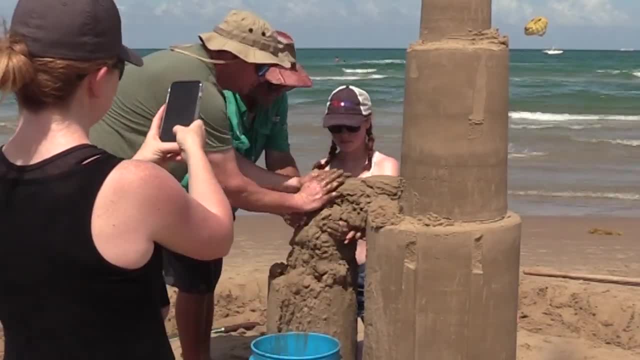 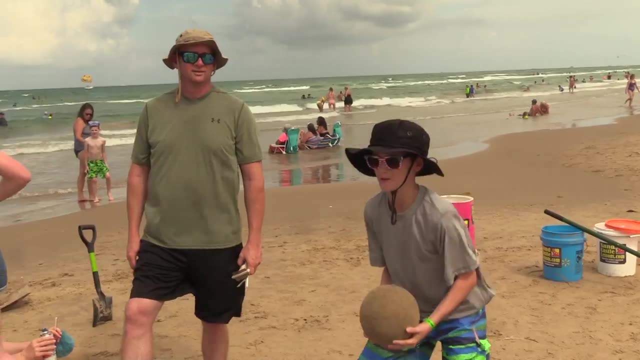 a tree on top of the mountain, just if you want to, the more technical way. but we put our informs on top so you can see this too, because we need the most stuff on the top and the small meters. so it's great, we're done. so, gosh, it looks so great. this is so simple. I àme out it's, i touch.